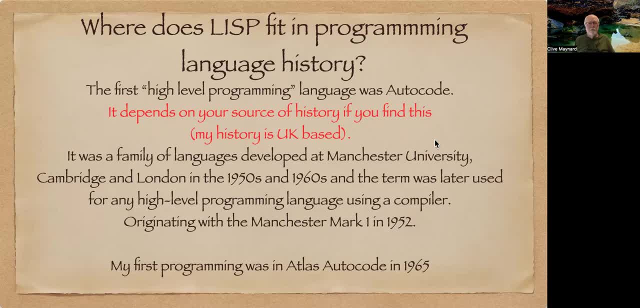 And it was originated with the Manchester Mark I computer in 1952. And I tie myself back that far by at least to 1965. Where I did some programming on the Atlas computer using Atlas autocode. Now, where does autocode fit within programming languages? 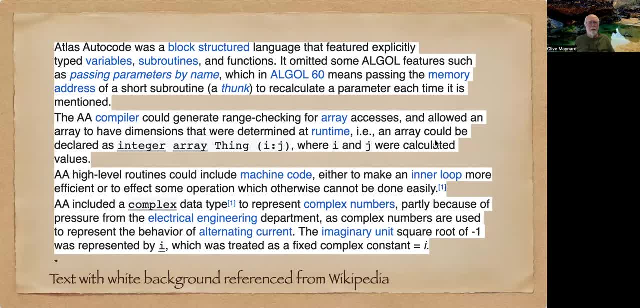 Well, just a couple of comments here: that it was related to our goal 60, but didn't have quite the same context, same contents. But a couple of the interesting things about it was it had arrays Which would be dynamic in the sense that you could determine the actual size of the array during execution, which was unique at the time. 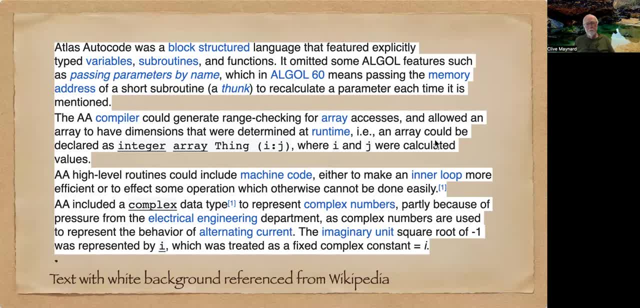 It was also the first high level programming language which actually had a complex data type, mainly from the needs of the electrical engineering department at Manchester. So it was a fairly sophisticated programming language. It also could directly include routines at the machine code level. 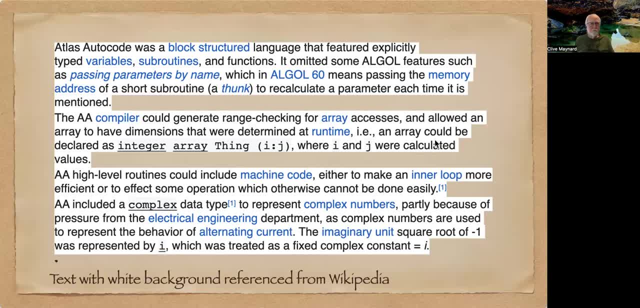 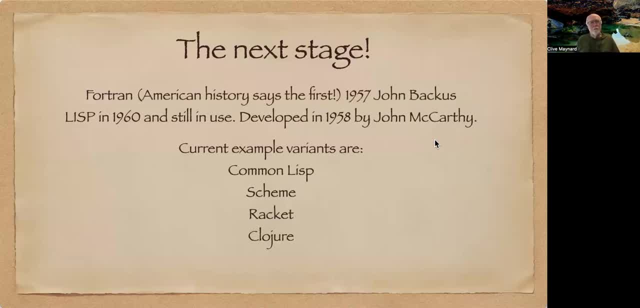 To get improved efficiency, So autocode was pretty important. If you, however, are looking at this from an American point of view, then Fortran will be claimed to be the first high level language, basically from 1957, which is about four or five years after autocode. 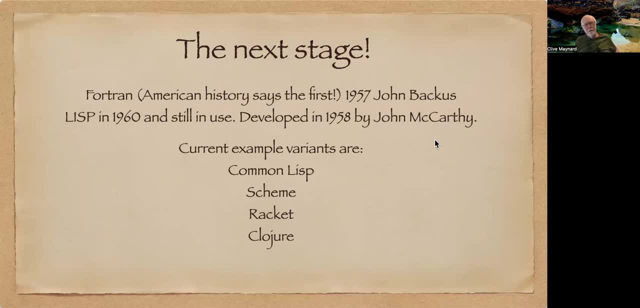 And then Lisp came along in 1960. And 1960s was way back. It was originally developed In 58 by John McCarthy but became known, if you like, in 1960 and and is still in use. And if you were to look around you'd see there are a number of current variants available. 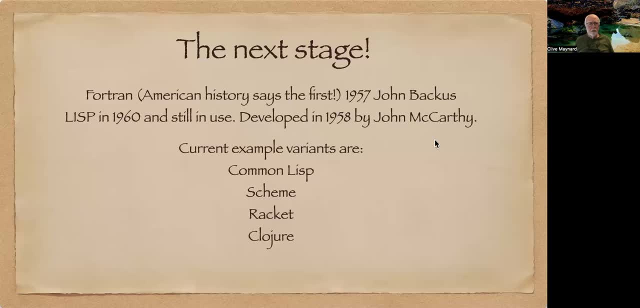 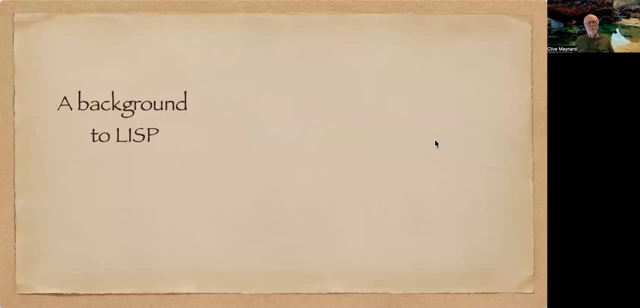 Common Lisp scheme which was from MIT Racket and Clojure. So let's give ourselves a little bit of background to Lisp here. So if we want to take an arithmetic expression, there are three notations to represent that expression which we can use. 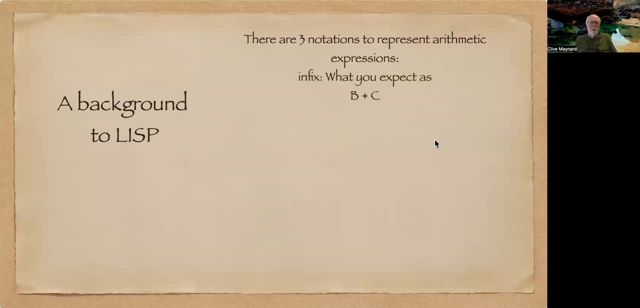 There is infix and what you would expect is that the operator, in this case the function being performed, is placed between the variables which are being computed. So B plus C, you get plus in between here. That's a very conventional environment. 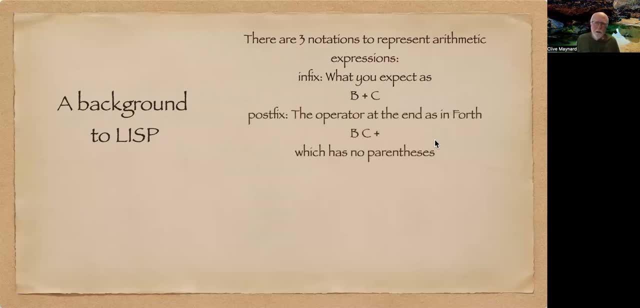 The second one is postfix, where this is where the actual operator appears at the end. the most well-known language in which this was used is fourth, and it doesn't need any parentheses, in fact. So you would have the value B, you'd take the value of C and then you would add them together to produce the result. 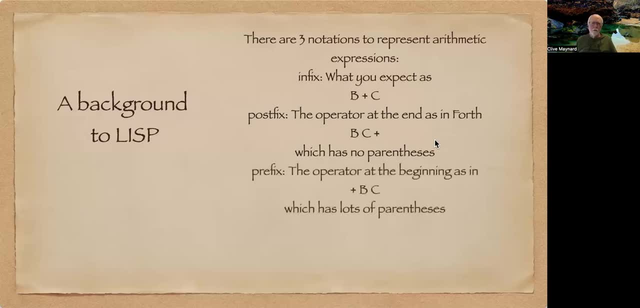 So no parentheses. Finally, there's prefix in which the operator is at the beginning, So in this case we have plus, That's the first one, Plus B and C. Now that potentially has lots of parentheses, because do you know where the end of the function is? 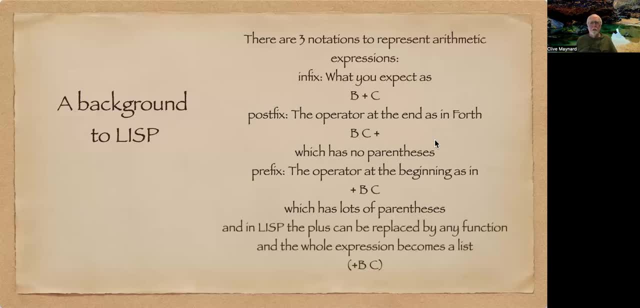 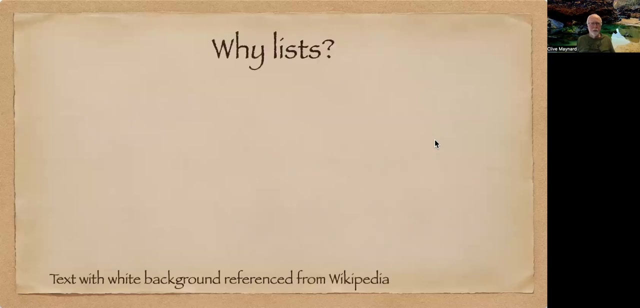 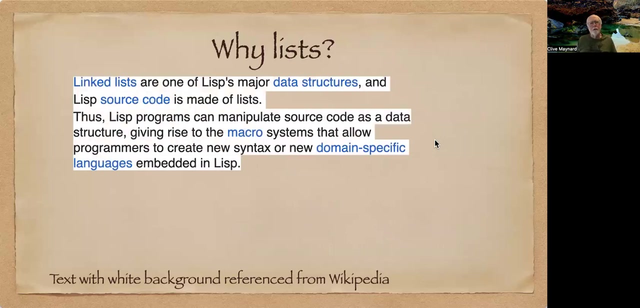 Possibly not So. therefore, in Lisp, the plus can be replaced by any function and the whole expression became a list. It was all put in a bracket, so you knew how far that operation was to be performed. So why lists? Well, it's basically Lisp's major data structures, or one of its major structures, and it really created a complete new syntax for representation of information and the programs. 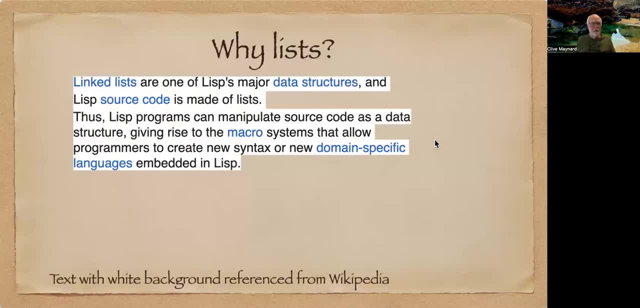 So the source code is also as a list, giving the possibility that you can have your program manipulate your source code. So the source code is also as a list, giving the possibility that you can have your program manipulate your source code. So the source code is also as a list, giving the possibility that you can have your program manipulate your source code. 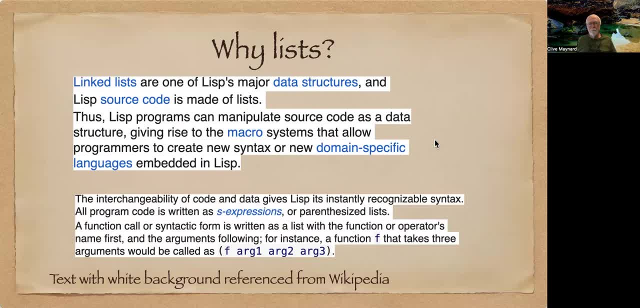 This interchangeability of code and data gives Lisp its differentiation, if you like, from others. Generally, a program is referred to as a set of S-expressions, or parenthesized lists, And in general any statement within Lisp will be of the form of as shown there. if you had a function F- it takes three arguments- then it would be brackets F, arg1,, arg2, arg3, closing bracket. And, in general, any statement within Lisp will be of the form of as shown there: if you had a function F, arg2,, arg3, closing bracket. And, in general, any statement within Lisp will be of the form of as shown there: if you had a function F, arg2,, arg3, closing bracket. 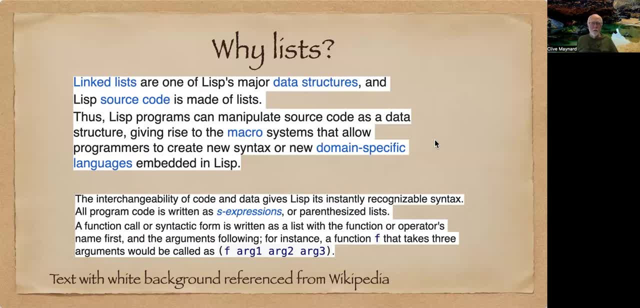 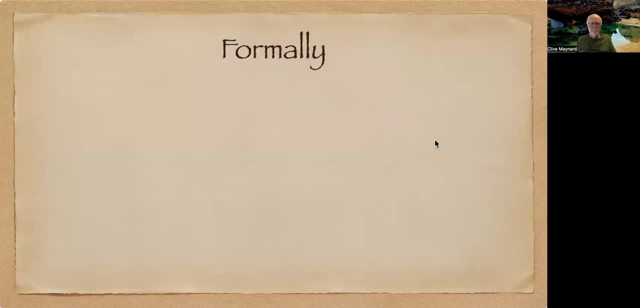 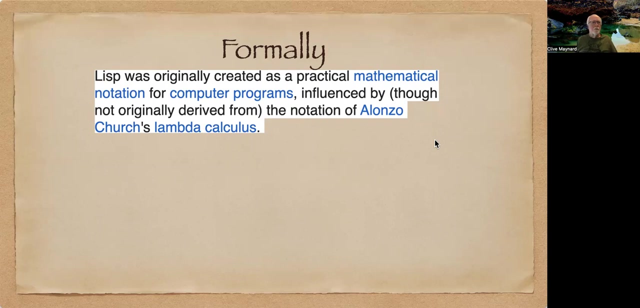 So that is a list and it is also a representation of a program within the Lisp context. So, from a formal viewpoint, where did Lisp come from? Well, when proposing programming languages, we go back as far as Alonzo Church's lambda calculus, which was the way in which you could represent an expression which could be computed. 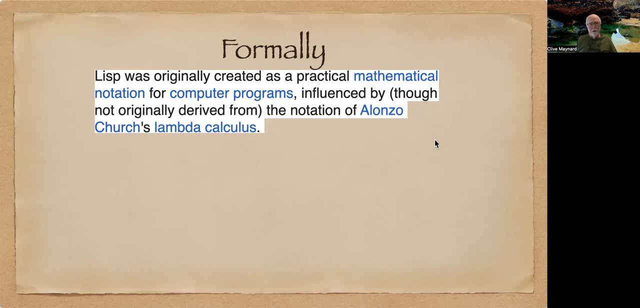 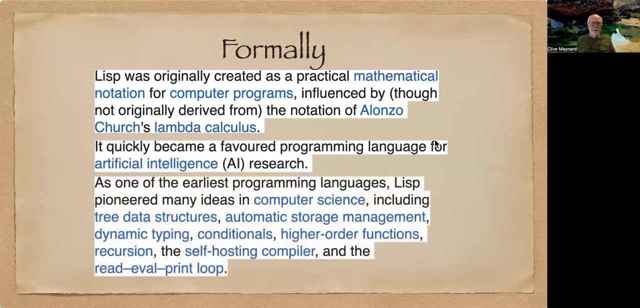 Using a Turing machine, And essentially, Lisp was the notation used in order to represent a lambda calculus, And so it quickly became a favorite programming language, particularly for artificial intelligence research, And as one of the earliest programming languages, it included many things which we now think of as standard, if you like. 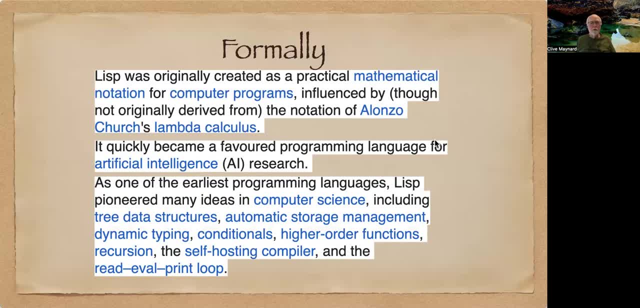 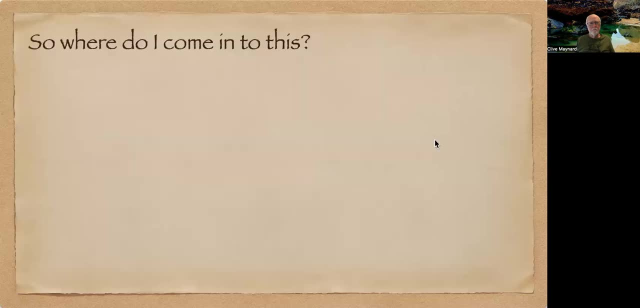 Tree data structure. Tree data structures, storage management, dynamic typing, high order functions, recursion- All of these things are considered quite normal within a programming language these days. So where do I come into this? Well, a gentleman by the name of Robin Jones, who was a university colleague of mine at the University of Canterbury. 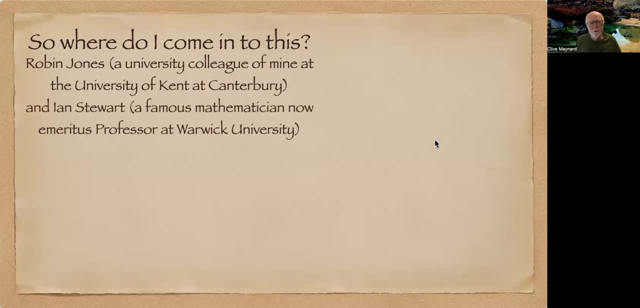 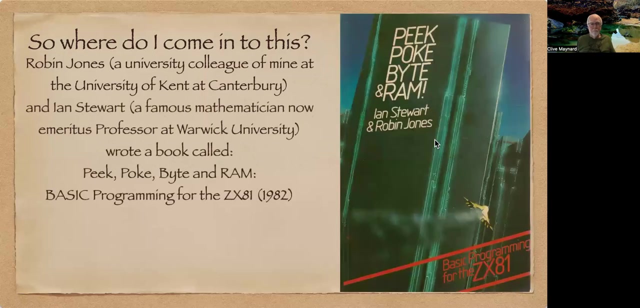 together with Ian Stewart, who I consider to be a fairly famous mathematician. he's now emeritus professor at Warwick University in the UK. They wrote a book which was called Peak, Poke, Pipe and Ram, And it was essentially basic programming for the ZX81, which was a small personal computer, one of the earliest. 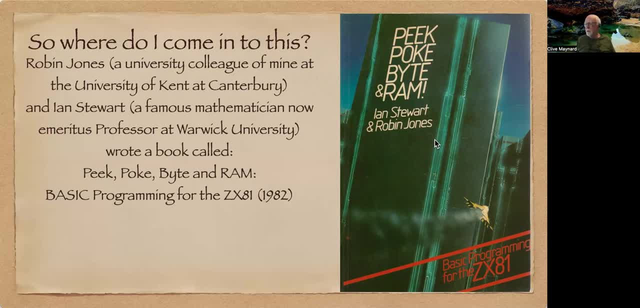 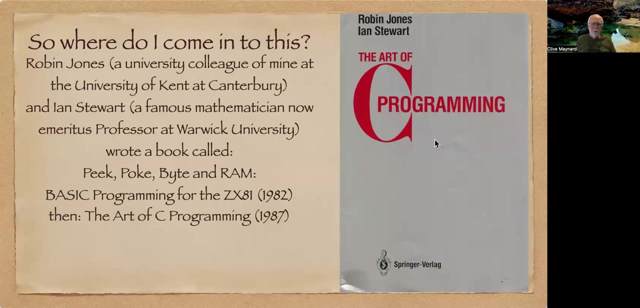 And it was actually quite successful And written for a British publisher. Later they were asked to go to a different language And they then wrote The Art of Sea Programming in 1987, the two of them- And they wrote it for Springer Verlag, a German publisher. 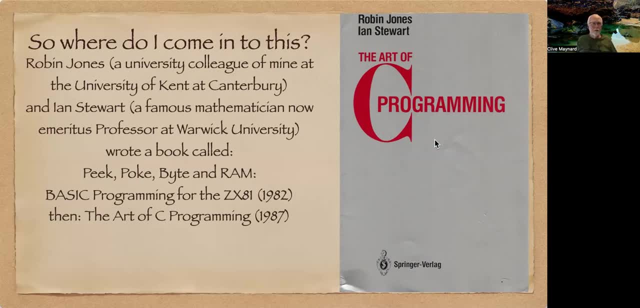 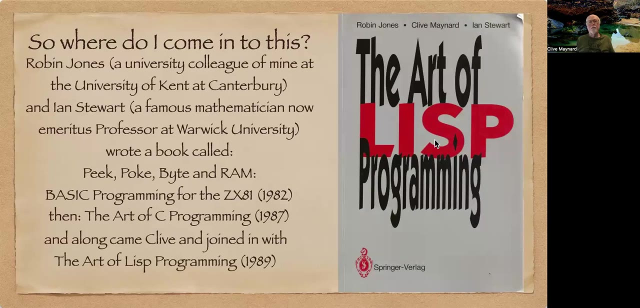 essentially with the aim of selling into the American market. And it was quite successful. So they were well established at this point. And Then along came myself. I was asked to join them And we wrote a book called The Art of Lisp Programming. 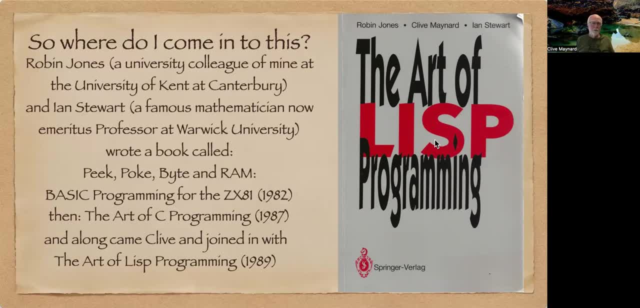 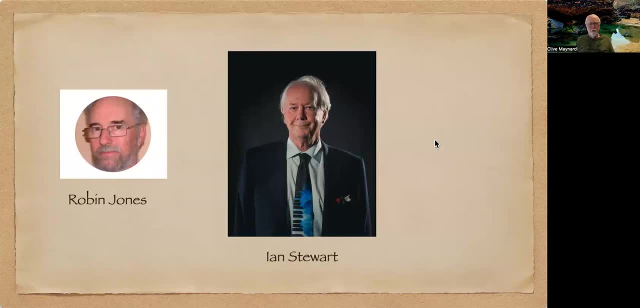 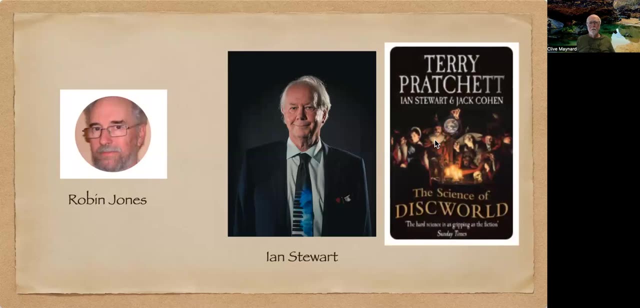 So that's where I get my first involvement seriously with Lisp. Now, Robin and Ian are shown here, But Ian is not only known as a mathematician. He is also known for having worked with Terry Pratchett, the author and involved in 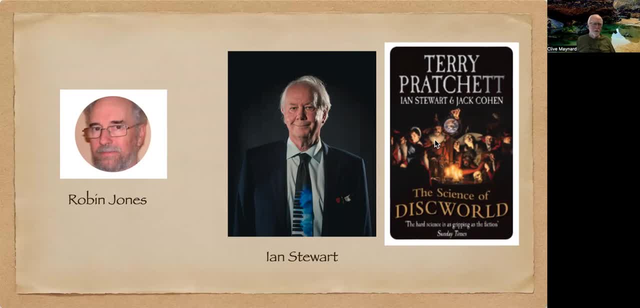 books called The Science of Discworld, et cetera- A whole series of books on that. So Ian has both serious mathematics and, if you like, enjoyable books as well, And so the three of us got together to write this book. 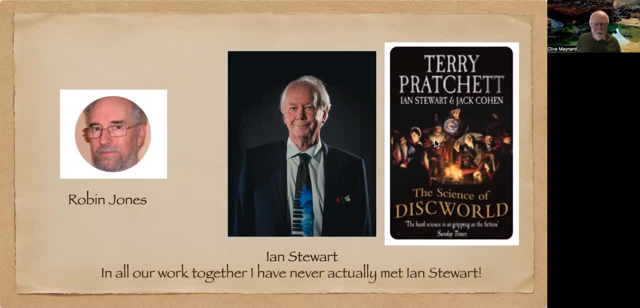 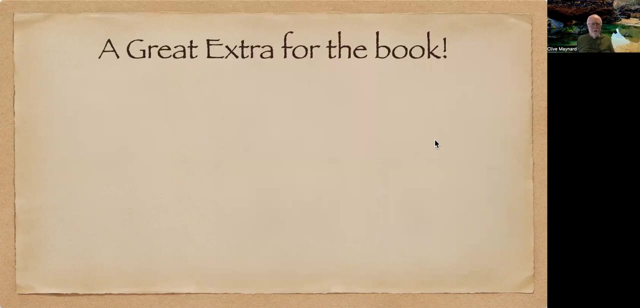 And when I say we got together, we worked ourselves together remotely And in fact in all the work we've done together I've never actually met Ian. We've only been in remote contact. Now let's have a little bit more on the book. 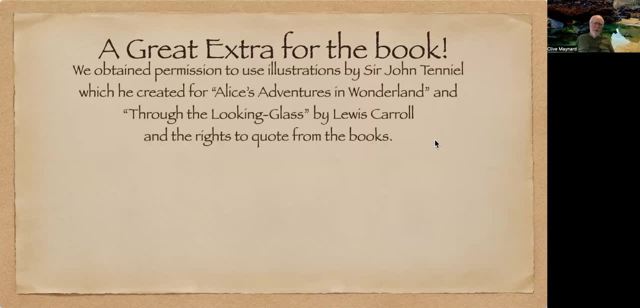 Well, we actually obtained permission to use the illustrations from Alice's Adventures in Wonderland and Through the Looking Glass and also the rights to quote from the books, And that was really good. It helped the structure of our book and it made it more enjoyable for the reader. 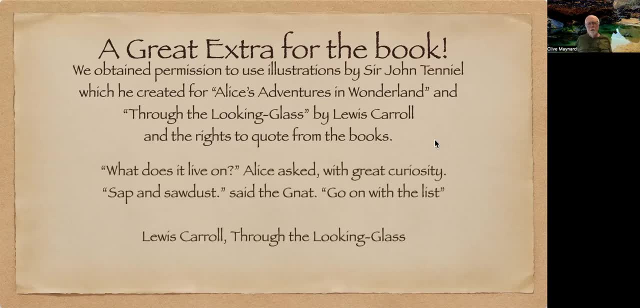 So, for instance, a quote there: What does it live on? Alice Asked with great curiosity. Sap and sawdust said the gnat, Go on with the list. And that was from Lewis Carroll, Through the Looking Glass. 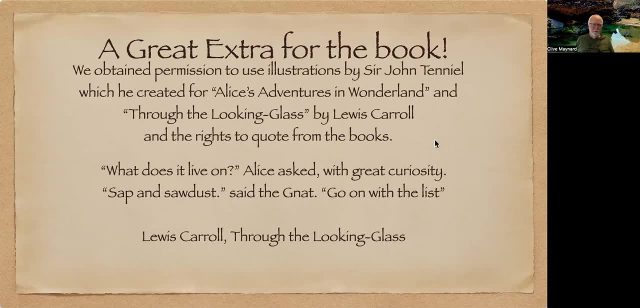 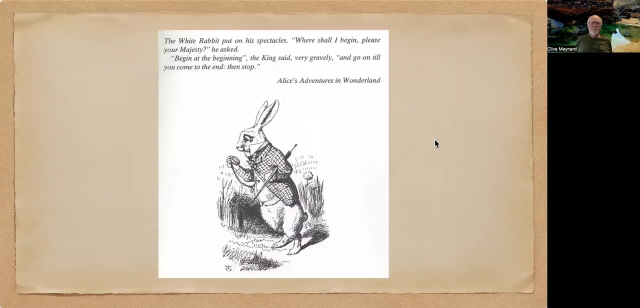 It's amazing how many good quotes and cartoons are useful from within those books. So here's one of the cartoons The White Rabbit Put on His Spectacles. Where shall I begin, please, your majesty? He asked, Begin at the beginning. the king said: 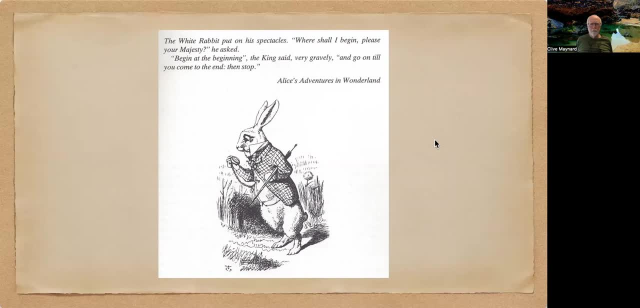 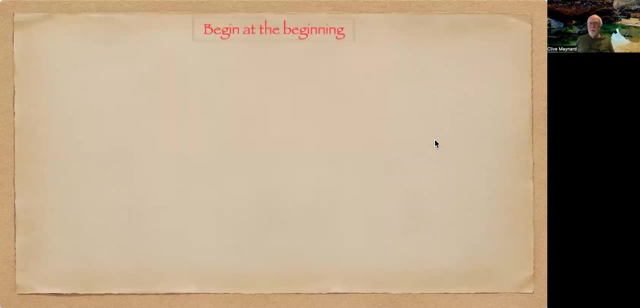 Very gravely And go on till you come to the end. Then stop. That's from Alice's Adventures, And so we will begin at the beginning. Let's start our journey into lists, considering how we might represent text as a list. 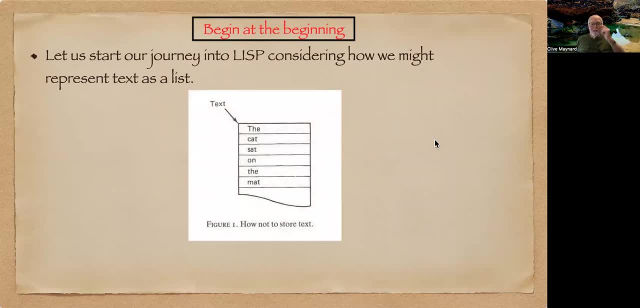 There are all sorts of formats you could use here, And this is a simple but not very efficient one. For instance, we had a A sentence here to represent, with the cat sat on the mat, And a block of memory is allocated to each of the words. 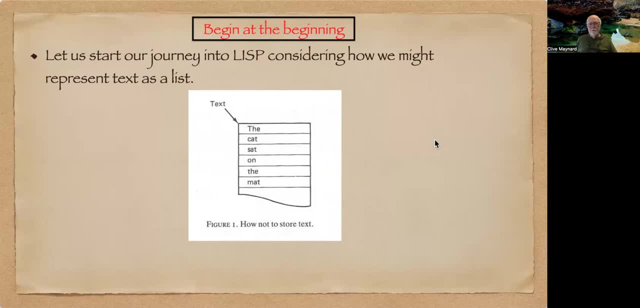 The amount of memory allocated was not, in this case, dependent on the size of the word, Though most of the words are only three letters anyway. But it's not. It is a way of representing textual information, but it's not very efficient. 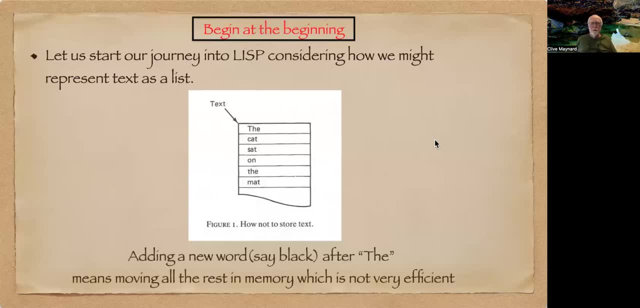 So what if, for instance, we want to, If we wanted to add a new word, so it became the black cat sat on the mat. It would mean that we'd have to move our array of words in memory, which is not very efficient. 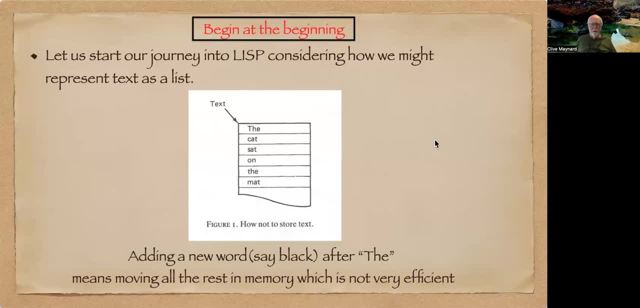 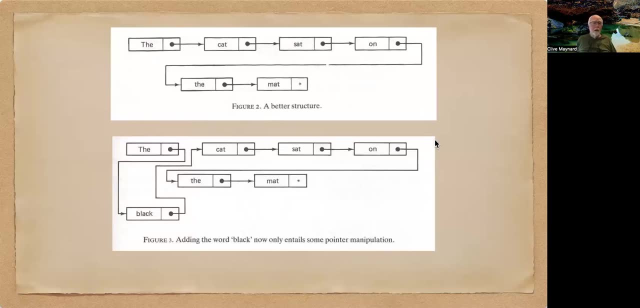 So can we represent text as a list in a more efficient manner? Well, looking at the top here we now have each word separate, but with a pointer to the next word in the sentence. So this is a pointer to the next word in the sentence. 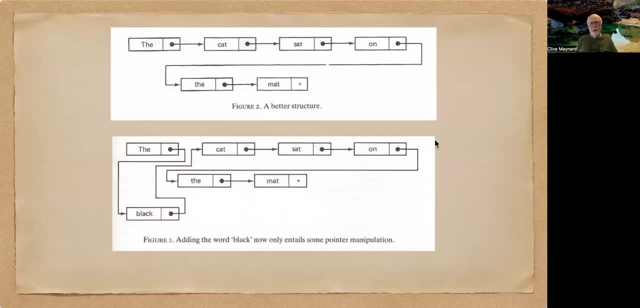 The is followed by a pointer which points to the second word, which is cat, with a pointer pointing to sat, et cetera on through the whole sentence and finishing with a nil pointer. Now, is this any better? Well, if we look at the picture at the bottom, the figure at the bottom, you'll see that if we now want to put in our extra word black, we simply have to change the pointer from the to the word black and from the end of the back back to the cat. 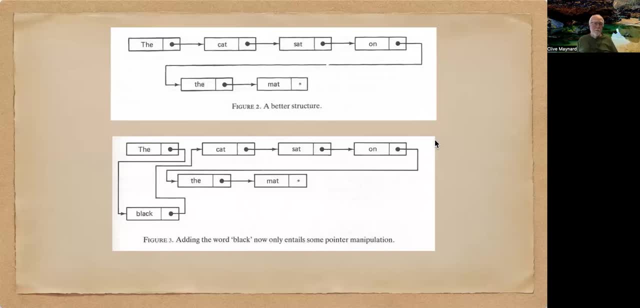 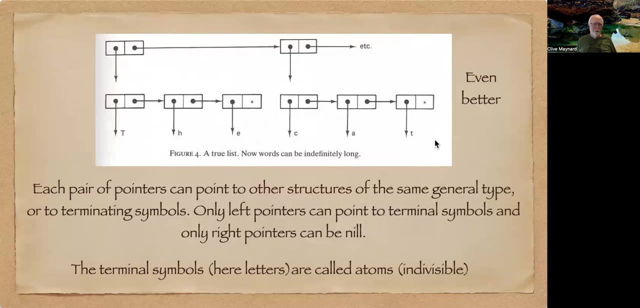 And without moving anything around, just by changing those pointers, we are able to add that extra word into our string. We can take this even further. We can make pointers a much more serious part of our structure. So this is even better from the internal representation point of view, but not necessarily from your point of view visually. 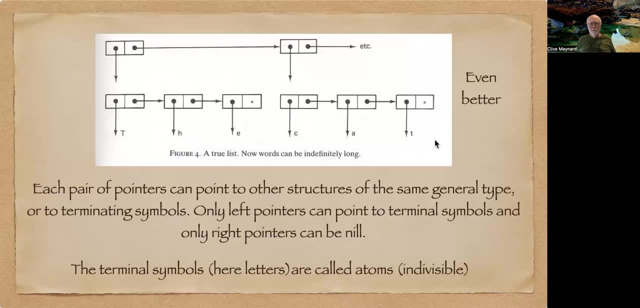 So we Everything is in pairs of pointers, and each of those pointers can point to other structures of the same general type or to terminating symbols. So, for instance, if we see the left-hand pointer which is pointing down in this diagram, it's pointing down to a set of three sets of pointers. 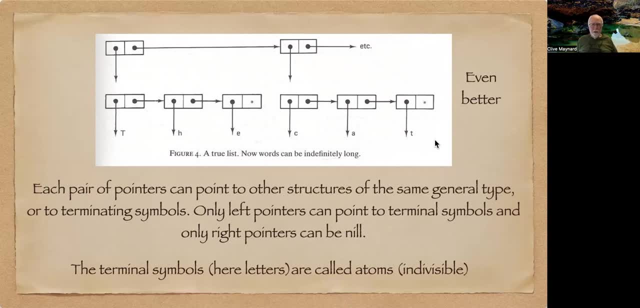 One goes on to the. Firstly it goes on to T, as a symbol, Then the next one goes on to H, The next one goes on to E And then there's a nil, So that's the. The word the is represented by that piece of the string. 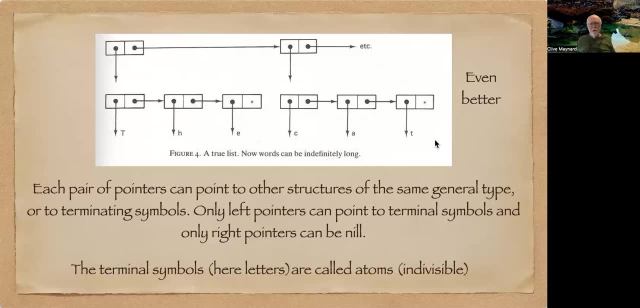 The right-hand pointer at the top points on to the second such string combination, where the left pointer goes down to the word cat and the right one goes on to the rest of the structure. So generally only left pointers can point to terminating symbols and only right pointers can be nil. 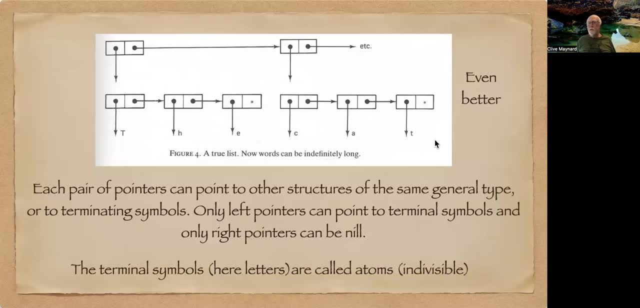 And where we do get terminating symbols, such as letters, we generally refer to, We refer to them as atoms within this context. Now, that's starting to look a little bit complicated and it's not in a form, of course, which we can start writing programs with. 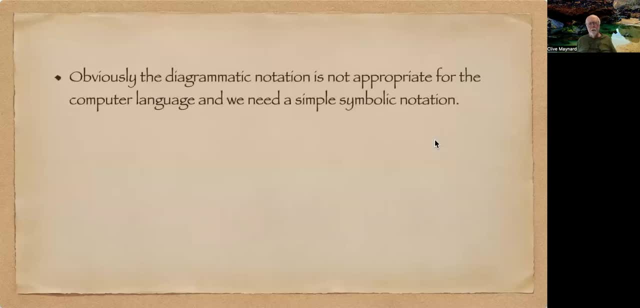 So we need to change the information. We need to change from our diagrammatic notation to a symbolic notation which will allow us to represent and manipulate the information within our strings. So, for instance, if we, If we had a list of letters A, B, C, D, it becomes written in our symbolic notation as in brackets: A, B, C, D. closing bracket. 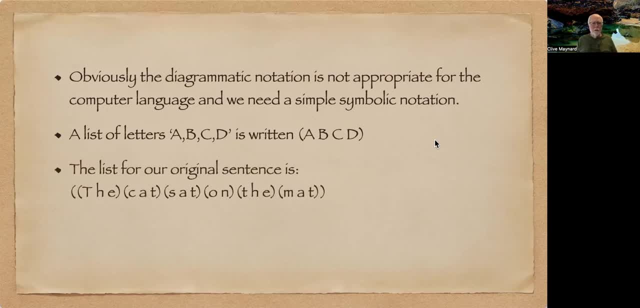 So for instance, for our original sentence it would be: And reading out makes it very difficult as you can see the infuriating silly parentheses. But if you say bracket, bracket, the closing bracket, open bracket, cat closing bracket, open bracket, sat. closing bracket, open bracket. 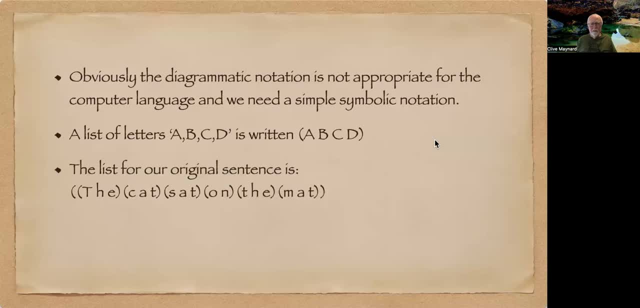 On, et cetera. So we can visually see it, We can see how our parts are defined And, of course, we can relate this back, if you wish, back to the diagrammatic representation which we had before. 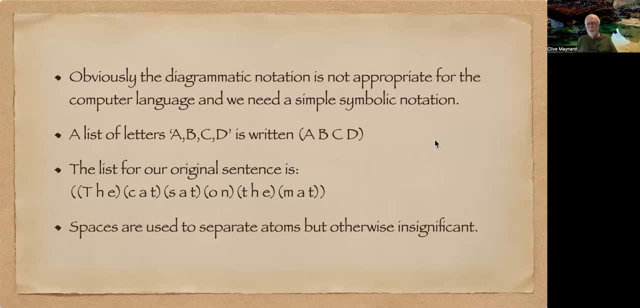 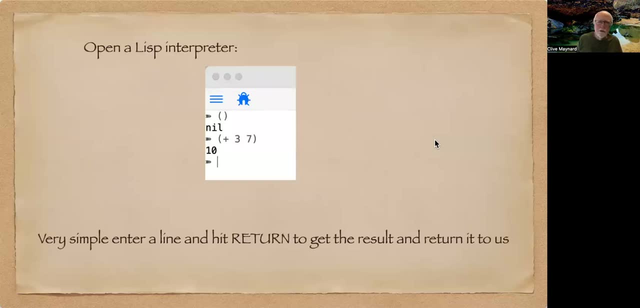 Generally consider that spaces were used to separate atoms, but otherwise were considerably insignificant. If you take your computer and just open a Lisp interpreter on it, We can very simply see how some things work. So for instance, if we just have an opening and closing bracket and hit return at the end there it'll just come back and say nil. 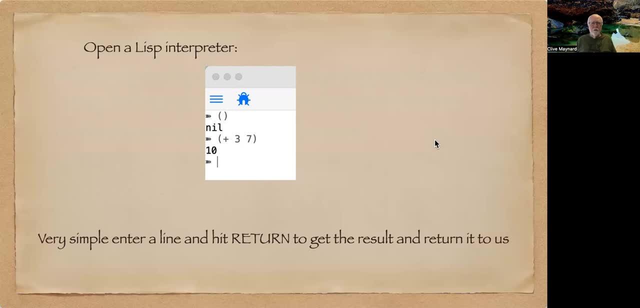 There's nothing in there. We don't have anything in our list. But if we did the bracket plus three, seven closing brackets- and hit return, we get the answer 10.. So we can see there that we're actually getting an operation done and a result is being returned. 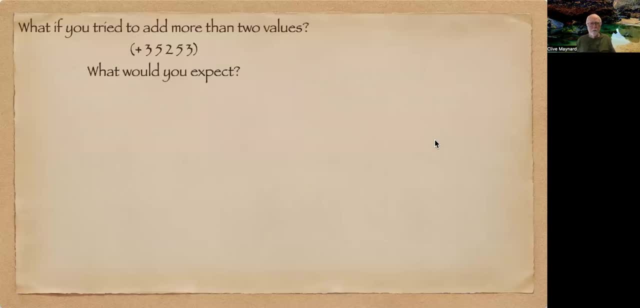 The result, The computation, is being returned in this context. So what if we tried to add more than two values? So here we're saying brackets plus three, five, two, five, three. What would one expect the Lisp processor to do? 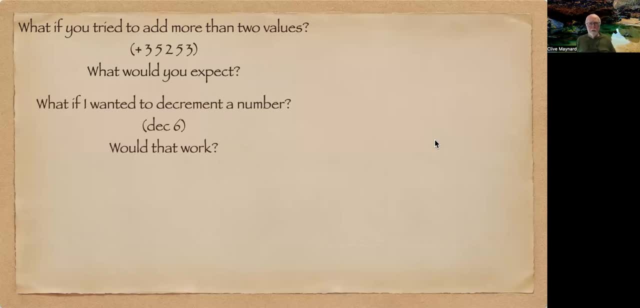 Considering another possibility: what if I wanted to decrement a number? So I decided there should be a function: dec, which, if we say dec six, Would it work? Would it give me an answer of five? Well, here we can see: if we do our plus three, five, two, five, three operation, we hit return, we'll get our value 18.. 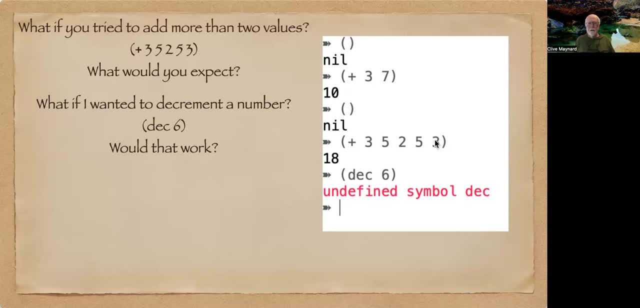 So what it says is that the plus function can take a number of arguments and it simply adds them all up. On the other hand, if we haven't really defined our dec function, it's not part of the core functions available. It will just come back. 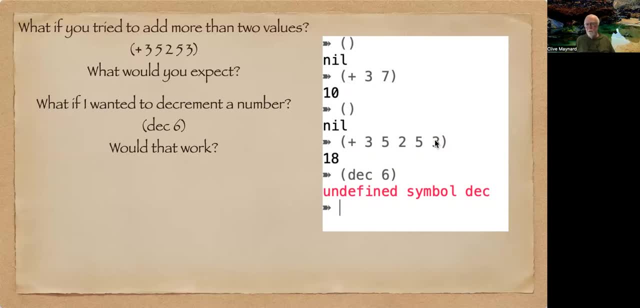 So I can say it's an undefined symbol, dec, and what's up to you to now make some definition of this. So the first thing we can say, then there are obviously functions that exist and also some that don't. So the important question then is: how do we create new functions? 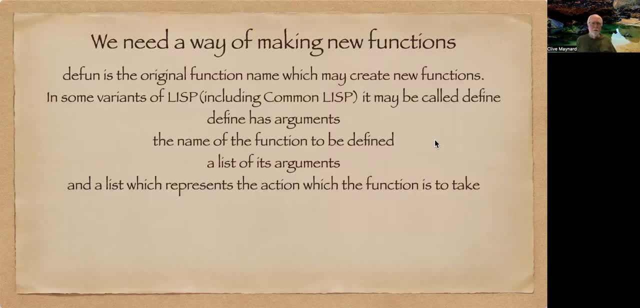 Well, the word for doing this- the function, if you like to write functions- was called defunct, But within the variations of Lisp became define, And so, in general now we consider the function define and it has arguments. The first argument is the name of the function which you're defining. 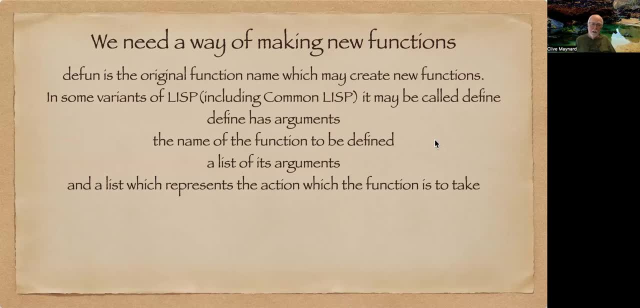 And the second is the list of its arguments, And then a list which represents the action which the function is to take. So, putting it into the context of our definition, we can say: here We're defining the dec function, So dec takes on an argument x. 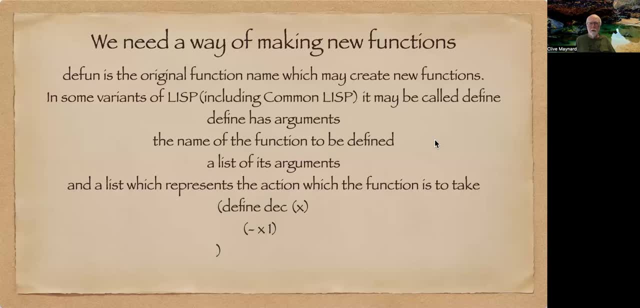 And what we expect to happen when we say dec of x is that we take minus x1, which is in brackets there. So it's taking the value of x, taking one away from it and returning whatever value you get. So we can now define a new function. 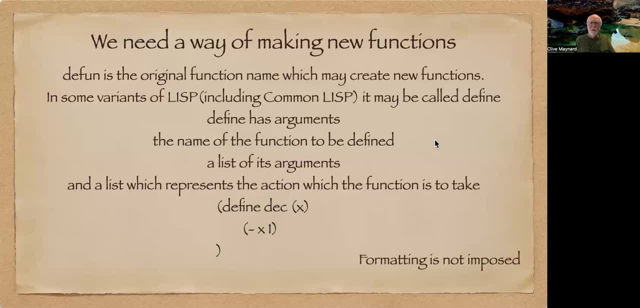 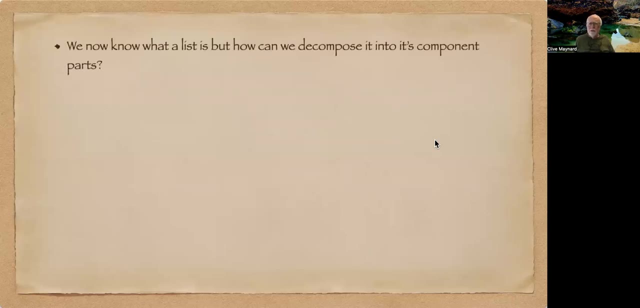 Notice this formatting which I've done here. It makes it easy to read, but it is not imposed within the language. It is not a compulsory part of the representation. So we now know what a list is, but how can we decompose it into its component parts? 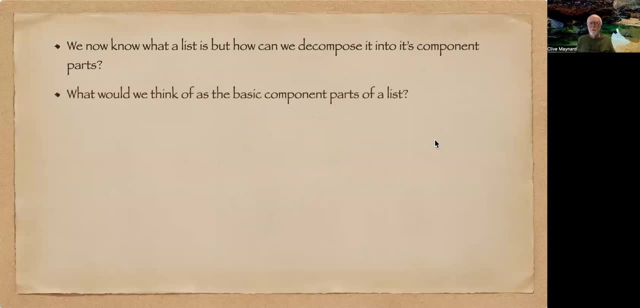 Well, what we need to do is to think of what are the basic component parts of a list. There's the first part of the list and you can consider the rest, So we have basically what we were calling the head and the tail. 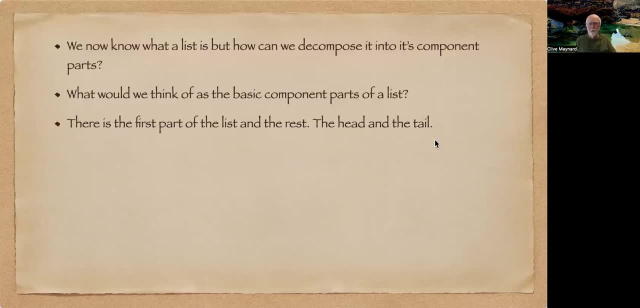 So we can have a function head which removes the first part of the list. We can have a function tail which returns the rest of the list. So if we had a list bracket, bracket a, b- closing bracket. open bracket c, d, e- closing brackets. 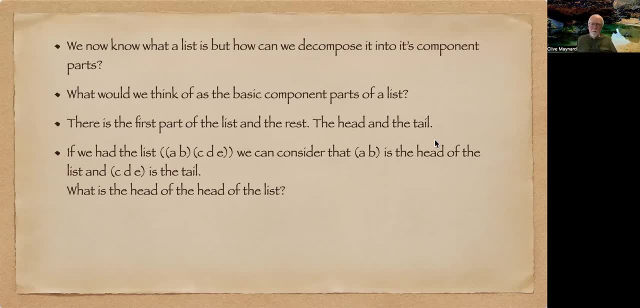 We can consider that a- the list, a, b- in brackets- is the head of the list and c, d, e is the tail For your own thoughts. what do you think of the head of the list? What would that be in this context? 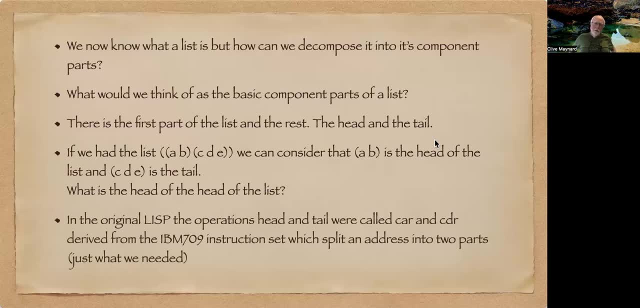 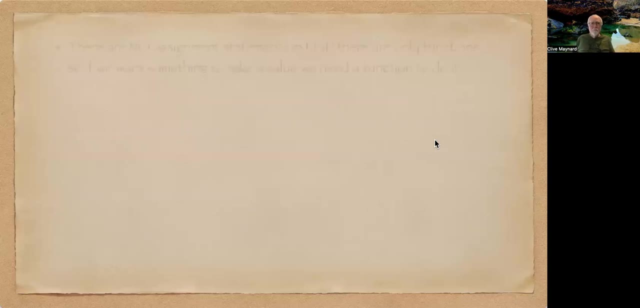 In the original LISP, these operations were actually called car and cutter, which were actually directly derived from the IBM 709 instruction set, which split an address into two parts, which is just what we needed for using our pointers. So, firstly, then, there are no assignment statements. 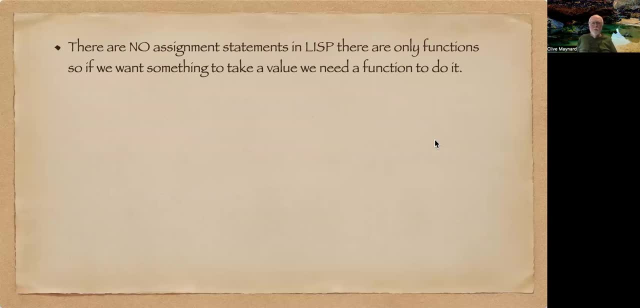 In LISP there are only functions. So if you want something to take a value, we need a function to do that. This is called a set quote. And I say for very specific reasons. we're not going into the depth here. 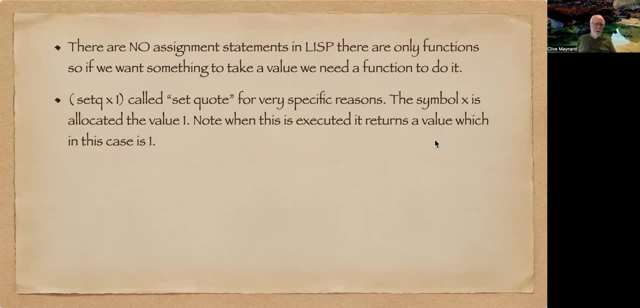 But the symbol x. in this context, if we say set, quote x1, is we take the symbol x and we allocate the value 1 to it. So when this is executed, it also returns the value, which in this case is. 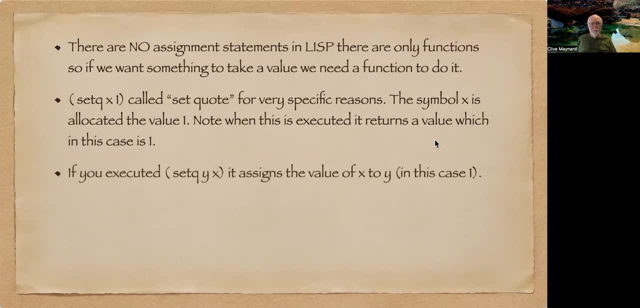 the 1.. If we executed set q, yx, it assigns the value of x to y, which in this case, is 1 from our previous definition. What if, on the other hand, we want y to have the value x, in other words, the symbol x? 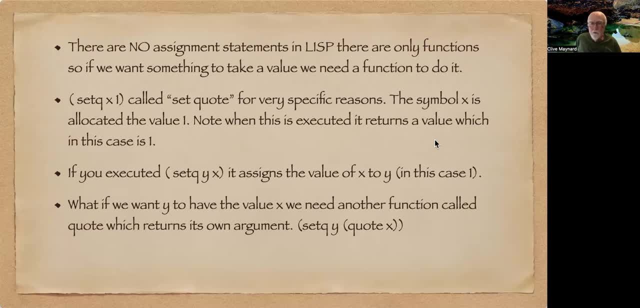 So we need another function which forces that process, And we call that function quote. And what quote does Returns its own. So we can now say: if we want y to actually be defined as being the symbol x, then we can say: bracket set q, y, then quote x. 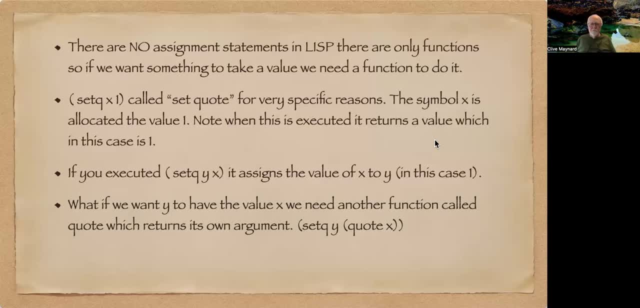 Now writing that out is a little bit, I don't know, takes too much work, Unwieldy. So there's a shorthand version of this where we just use a quote mark in front of the argument there. So we have set quote y, quote x. 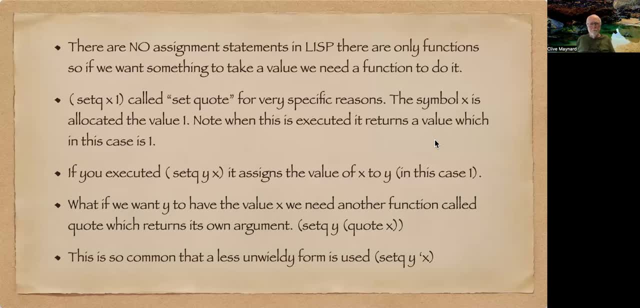 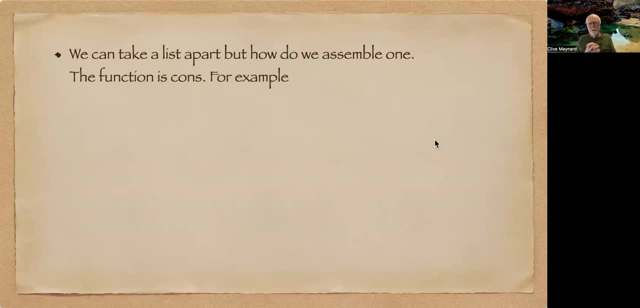 And it's written with the inverted comma. So where are we getting to? We can now take a list apart, But how do we assemble one? This is the opposite process And function in this case is called comms. So, for example, if we had set quote: h is a. 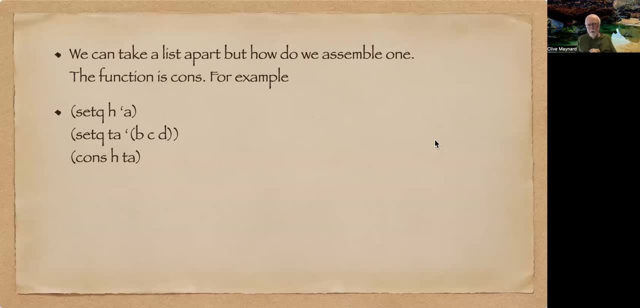 and set quote: ta is bcd- I should have said quote bcd- then the comms, the comms of h and ta, simply produces the list abcd. So we can take things apart, we can put them back together again. 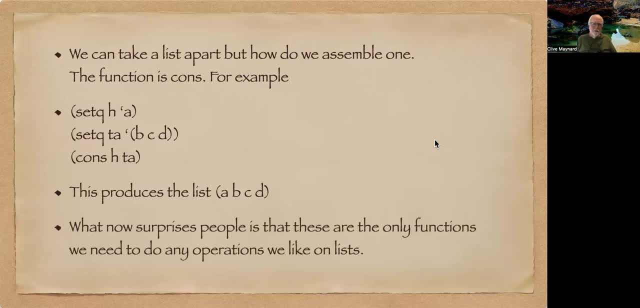 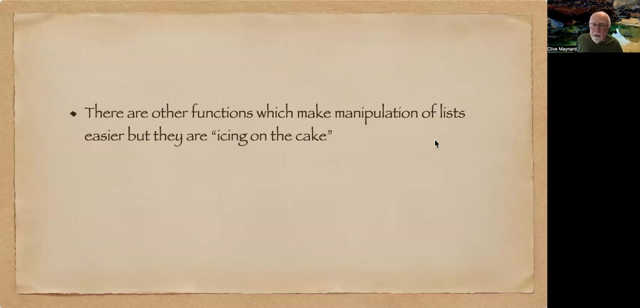 What surprises a lot of people when they start looking at lists is that with these and only these functions we can do anything we like with lists. It's a very surprising thing. We don't need a lot of complexity. The other functions we have for manipulating lists. 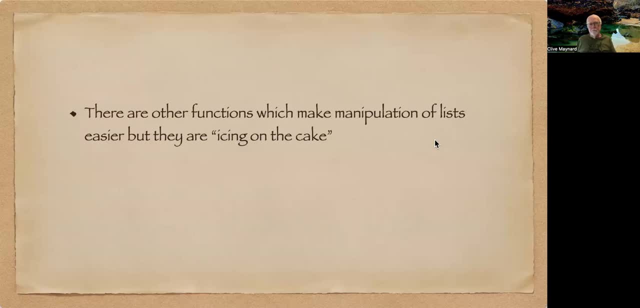 are simply icing on the cake. Extra functionality, Now, what I've done now is given you the entry point into the list, But I'm not going to go much further in this case. So, as I said here, I don't wish to overstay my welcome with this. 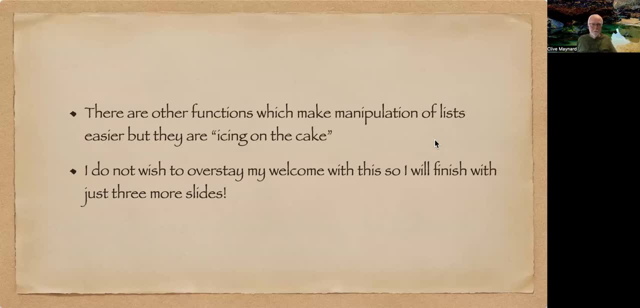 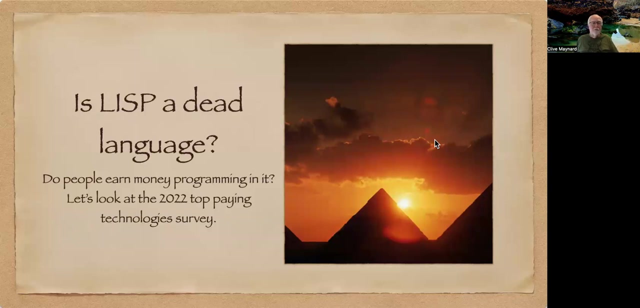 So I will finish with just three more slides And go on until you come to the end, Then stop. So we've been talking about lists. Is it something which is worth looking at? So is it a dead language? Probably the best way of measuring that, in a sense.